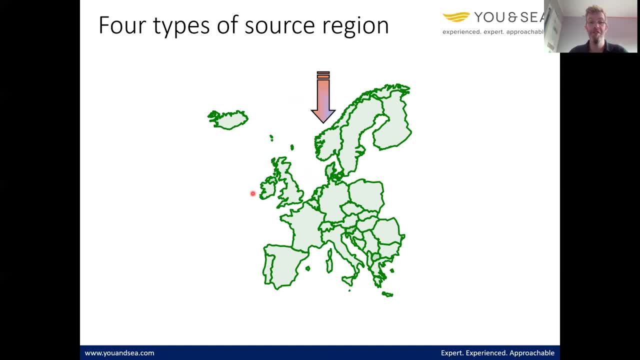 it for a minute. Let's look at four different wind directions: north, east, south and west. From the north, we've got the UK. From the south. we've got the UK From the north. we've got the UK From the north. we've got the UK From the north. we've got the UK From the. 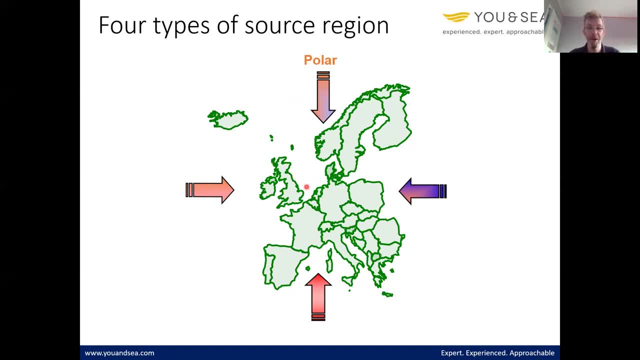 south. we've got the UK From the south. we've got the UK From the south. we've got the UK From the east. it's continental, From the south it's tropical And from the west it's maritime. It will be really straightforward if wind blew from one of those four directions. 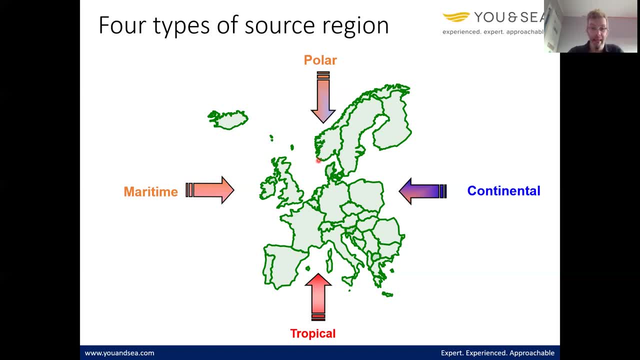 and that was it. But it's not So if we're going to take polar, it's cold, it's dry dry. although there is vast amounts of water, up at the poles it's all frozen, which means there's not going to be much rain. however, that in turn creates its own problem, because what we have with polar 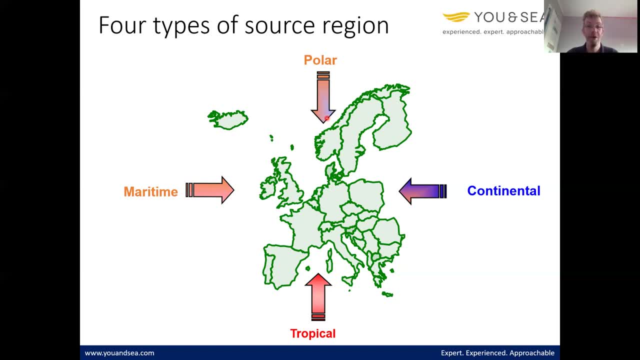 wind is cold air which, when it meets the warm, moist air that comes up from the tropics, we get snow. think beast from the east scenario: a northerly wind, even in the midst of summer is rarely warm because the Arctic is still there and it's still cold and it's still 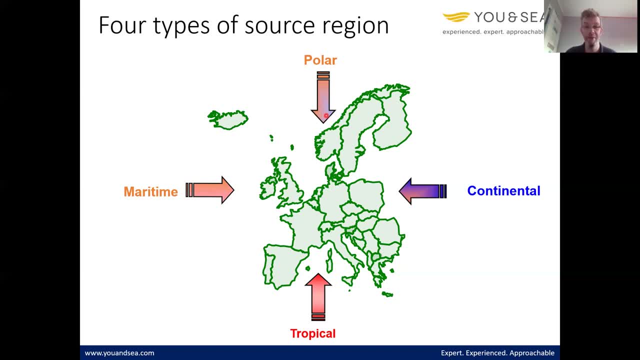 frozen. so all the air that drives down from the north is going to be cold. the continental one, easterly one, that changes quite significantly by the time of year. again very little moisture because it's from the continent. there's land, there's very small amounts of water and there's no air. so it's veryeled on the continent. so there's a very small 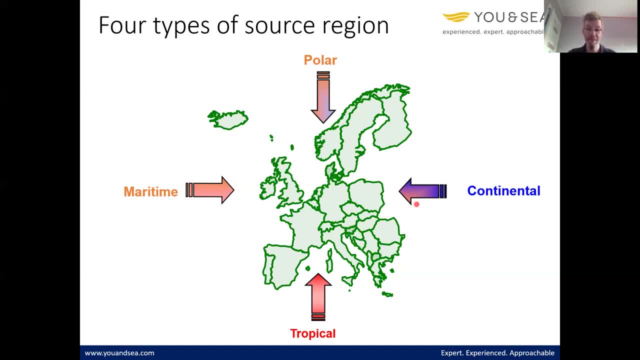 water for it to move over. it's going to be relatively warm in the summer. i think dubai kind of middle east and all the heat that comes from there, but equally it's going to be quite cold in the winter- tropics. that is going to be warm 12 months of the year. the reason it's tropical: 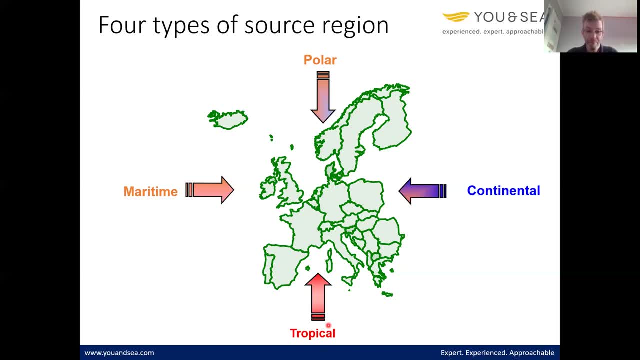 is it? as i just alluded to, it comes up from the tropics, which are always warm no matter what time of the year we are in. and then the last one is maritime. that comes from anything to do with water. so west of this little icon, we've got a few thousand miles of water, north atlantic for it. 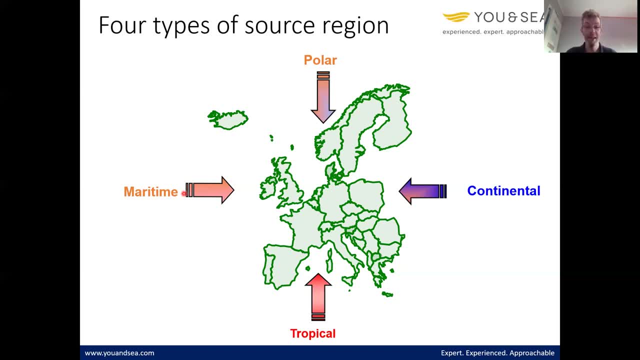 to be picked up and pretty much dumped in the uk, and that's one of the reasons why our uk weather is so changeable, because the wind direction shifts depending on what's going on. when we start to combine these two polar maritime, we get cold and wet weather. 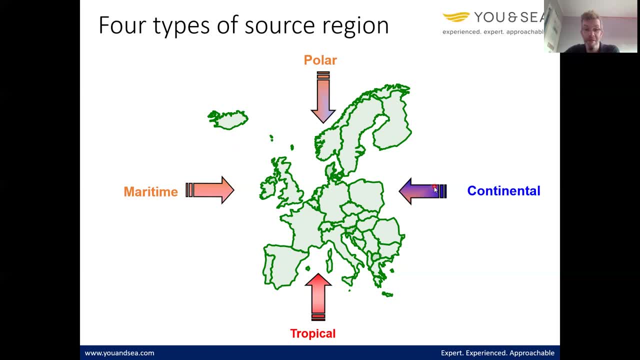 polar continental is just cold but relatively dry, and tropical continental doesn't tend to do anything other than put a lot of heat um into what we've got. but it's really going to tropical maritime that it starts to get a little bit kind of more interesting. reason being is southwesterly wind is the most common wind direction. it's the prevailing wind. 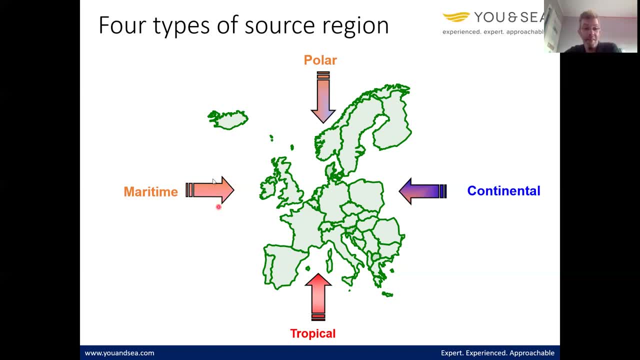 in the uk and that's going to combine all the moisture from from westerly with the heat from a southerly wind, so it's warm, moist air getting pulled out from the tropics in the equator, picking up all that moisture and then dumping it on the uk. 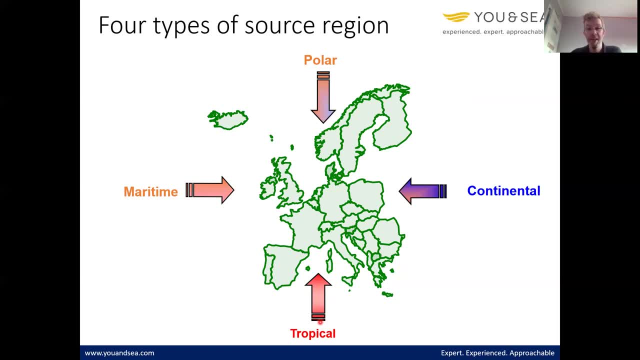 okay, certain parts of the year. you can get at least a 10 or 12 degree temperature change one day from the next. if it blows northeasterly it's going to be really cold, and if it switches around to the southwest, the temperature will increase by about 10 or 12 degrees. but sadly for us that's probably going to mean a warmer day. 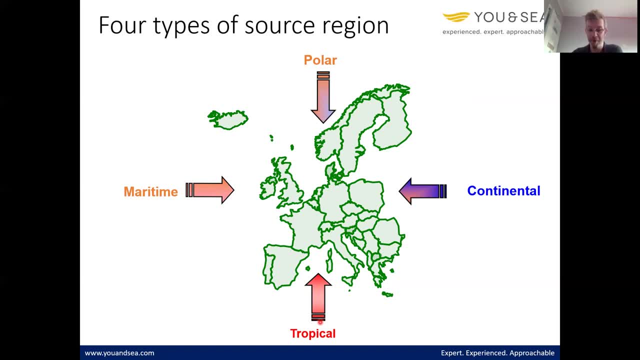 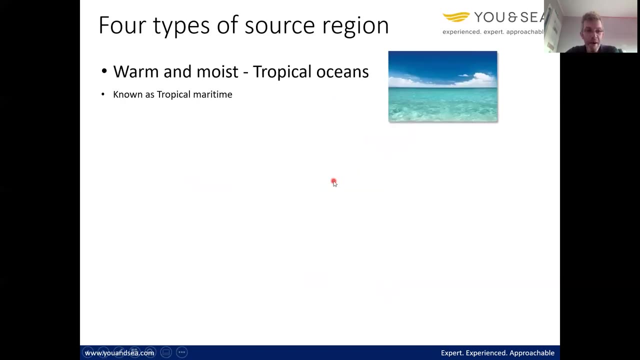 which is great, but lots of rain as well, and we'll go on to why we get lots of rain from southwest a little bit later on. so a little bit of a recap on what we've just done. so warm and moist oceans, that's what we call tropical maritime, warm and dry from the desert regions, the sahara. 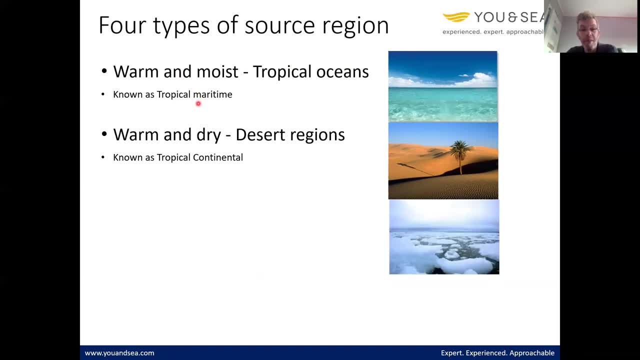 tropical, continental. i'm just staying with this for a second. this is: this is the reason that we get one of my favorite types of weather, and on the theory courses we get a lot of weather running in the classroom, i quite often get people to list as many types of rain as they can think of. 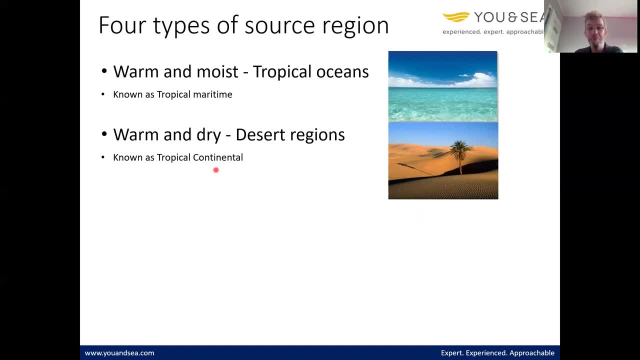 and very few people come up with dry rain, and a few uh that do know exactly what i'm talking about and everyone else uh thinks i'm better nuts, but we do get dry rain. it's obviously not wet because there's no moisture in the air, but the dry rain is what's in this photo? here it's sand or 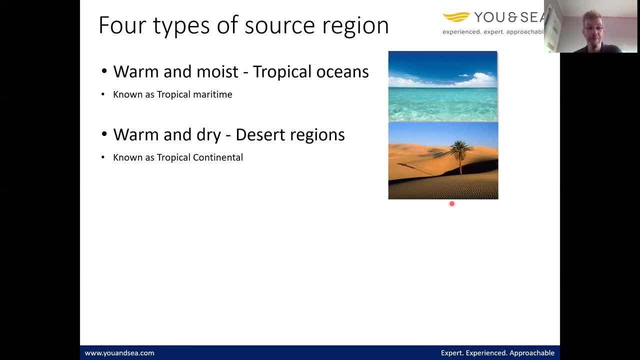 or very similar um kind of types and that will just get picked up with the wind and moved all across southern europe. used to be very common in greece. most of the southwest of the uk will get some kind of dry rain at some point, um, and it will put the cars, kind of bins, windows, um, like a very fine kind of dust. 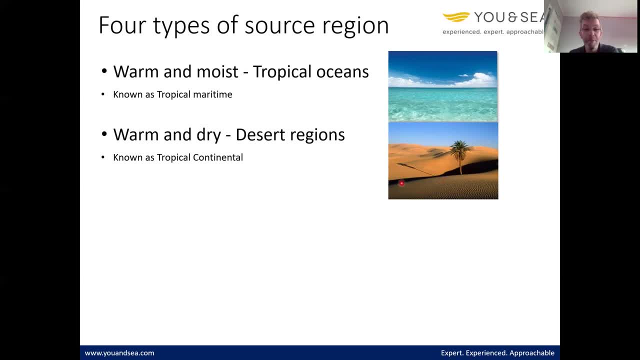 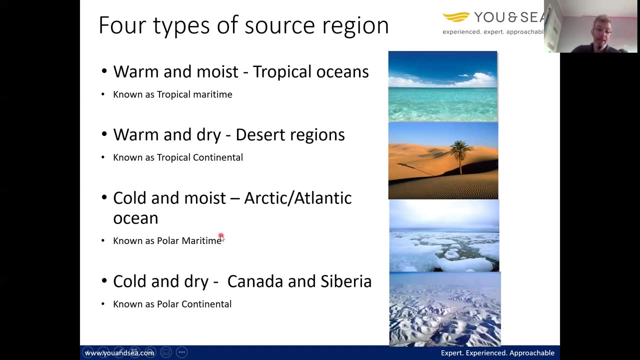 and it does turn everything kind of sandy color- quite rare but it does happen- cold and moist, from the arctic, the atlantic ocean, polar maritime could just bring kind of sleety conditions but equally could bring quite heavy snow. and then the last one, polar, continental, if we combine the first one, tropical maritime, with the 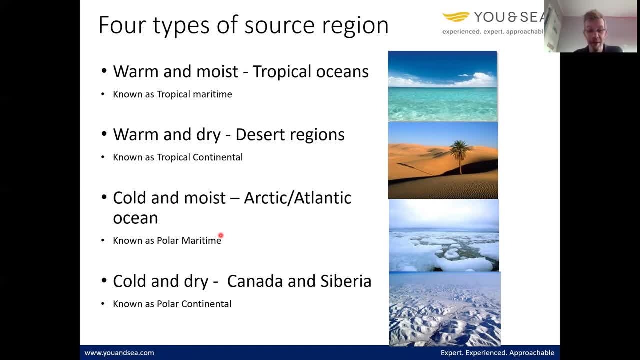 fourth one: polar continental. we've got what we encountered as beast from the east a couple of years ago. we had polar continental northeastern east meeting tropical maritime southwestern east, and the boundary between that weather was right down the middle of the uk, which is why we had a lot of that snow. 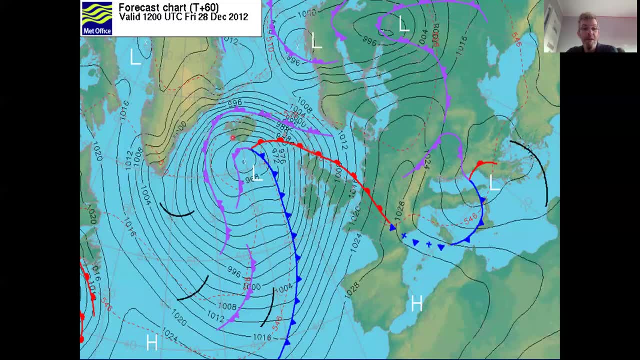 so this is what it all comes down to. this is a kind of simplified version um, with all the add-ons around the outside cut off. this is an optic chart um from a few years ago, so december 2012. things to note: we've got a low pressure. 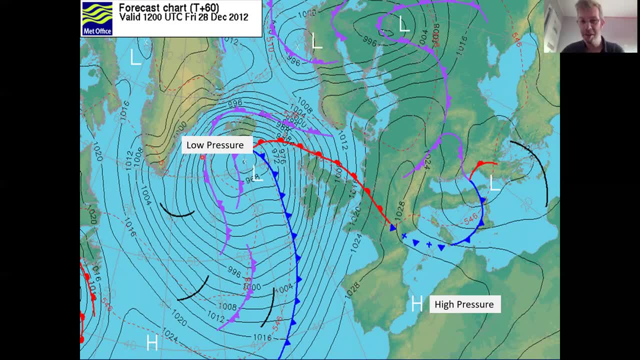 and we can always find the low pressure on a synoptic chart because it's accompanied by red lines, which are long fronts, blue lines, which are cold fronts, these purple wavy lines coming off it occluded fronts, that's where the two combine, and normally a large amount of black lines with a load of numbers on them are really kind of tightly packed together. 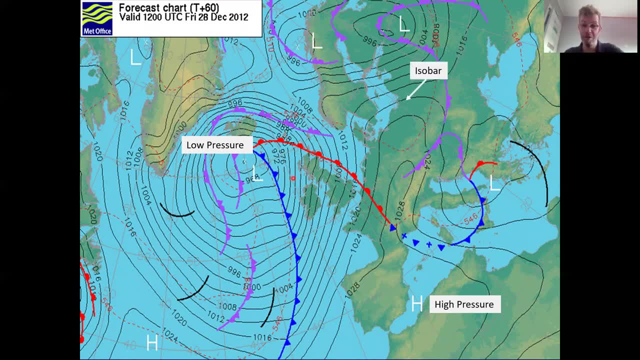 these black lines are what we call isobars, and we'll come on to what all this means in detail a little bit later. on. nice big high pressure down here. this is the european high pressure and it's always there. it just moves a little bit further south in the summer. 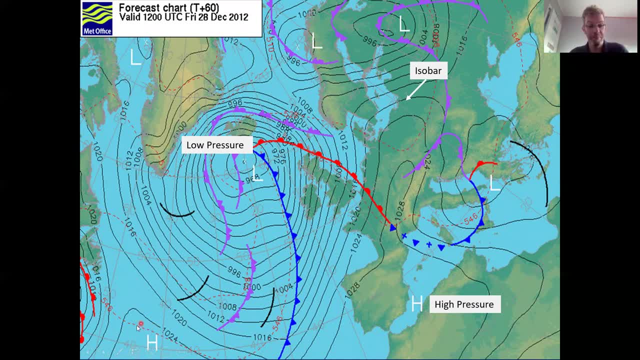 and we've got a little high pressure poking up here from the bottom left hand of the screen- the azores high pressure- and that stays there as well. it just moves a little bit further north or south depending on the time of the year. So the winter it gets pushed down and the 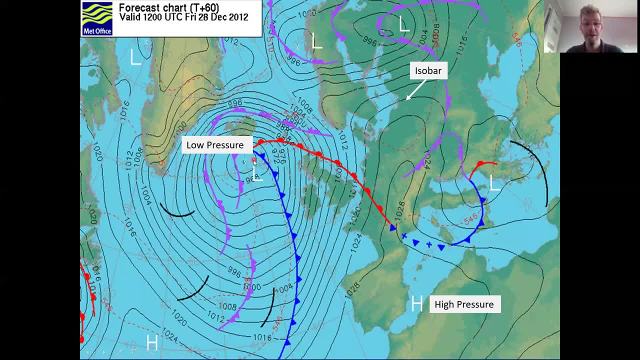 summer it starts creeping up towards us. So low pressure, high pressure isobars. The red warm front is the boundary, it's the meeting point between the colder air over here on the leading edge and the warm air in behind it here, And we call that. 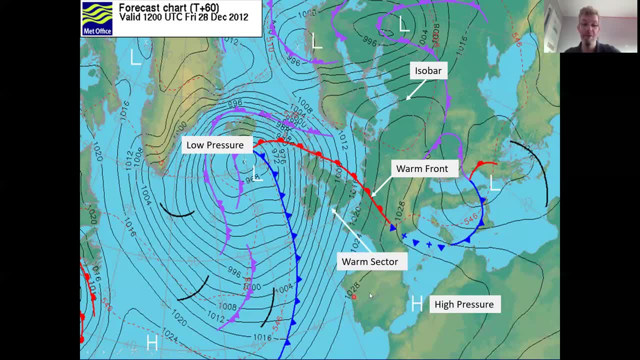 the warm sector because it's a little segment of warm air. We've got the cool front and this is the boundary, the meeting between all the warm air in the warm sector and the cooler air moving in behind. The way to think of fronts are essentially battlegrounds between 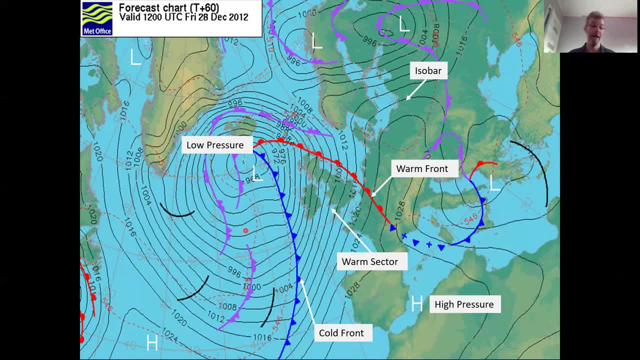 two air masses, Surrey the Gol, to have warm air and cold air, and the two of them are constantly going to battle, join, move. When we get a warm front, it means the warm air has won the battle and we get a cold front, the cold air has won the battle. 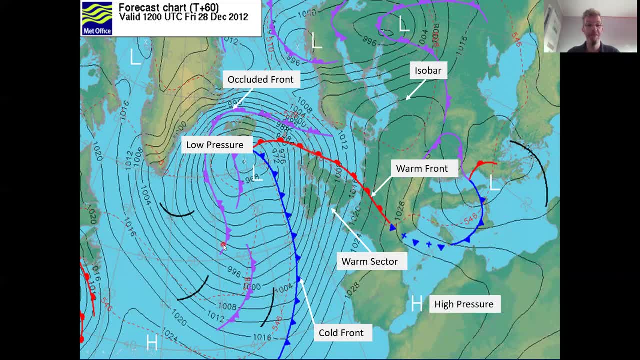 This last section over here that we can pick up from this chart is an acclimated front, and that happens in two particular areas. One on a low pressure, when the warm front and the cold front essentially zip up and join together and then the characteristics will will differ. I tend to refer 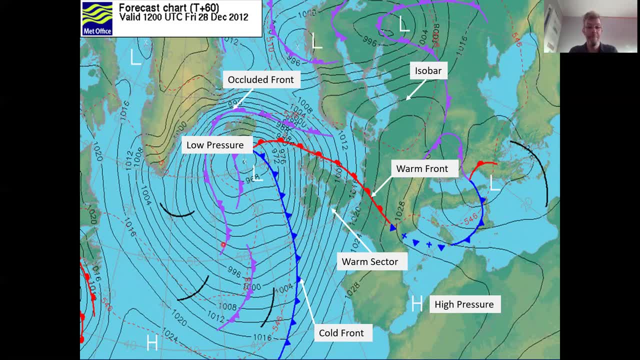 in some of the theory courses. if you imagine a line and you've got a cold front at one end and you've got a warm front at the other, that occluded front will take on the characteristics of those fronts, depending which end of that line is on. So if it's more of a kind of a warm front, 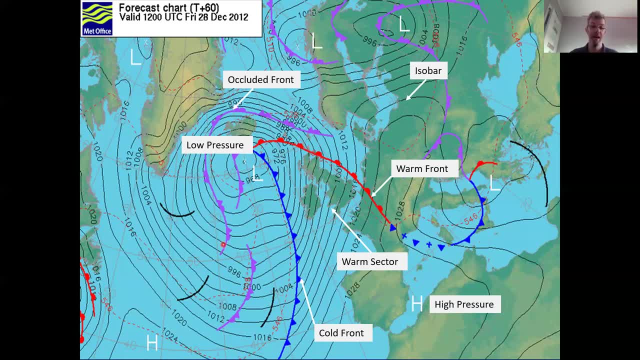 occluded front, you're going to have more heavy, persistent rain, and if it's more of a cold front type occluded front, then it's going to be more kind of isolated squally showers, And if it's in the middle, well, it could do either. 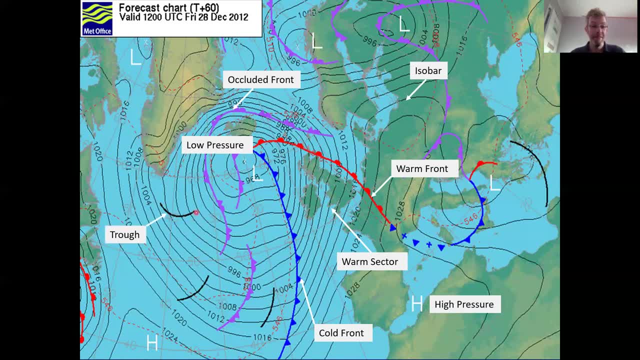 And the last thing that we can tackle here and identify these little black lines, and there's a couple of them dotted around. There's three in the Atlantic and then there's one over towards the eastern end of the Med and Aegean. So these little black, 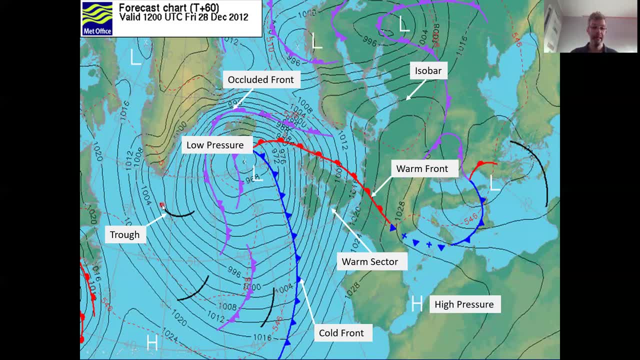 lines are what we call troughs. Very simply, we think of them as a very localized, deep area of low pressure. They bring in characteristics within a kind of a low pressure, wind and rain, a bit more of a kind of a serious squall, and then it'll clear off and it will move away. 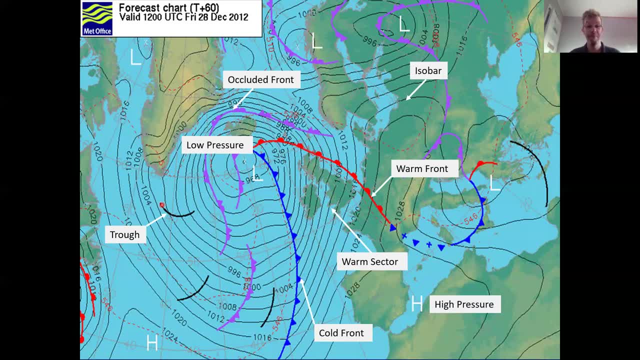 Really hard to forecast, really hard to predict where they're going to be, but they do get scattered around a snoptic chart from time to time. So, looking at a snoptic chart, we should be able to identify a couple of things. The one big thing that stands out for me, besides where the fronts are, is where. 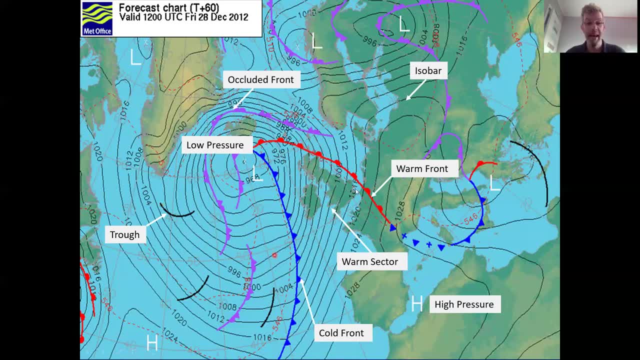 it's going to be windy and where it's not, And anywhere around this low pressure system, it's going to be windy because the ice bars are tightly packed together, And on this high pressure system down here, the ice bars are not tightly packed together, so we're not going to expect very much wind. 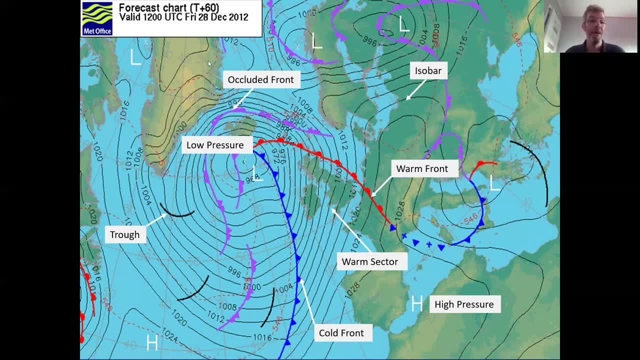 The third thing I can identify- and that's just bear with me while I bring up a kind of a marker, a yellow- Okay, that's wind direction that we're running going to get. I can identify that because of where the fronts are pointing. We've got. 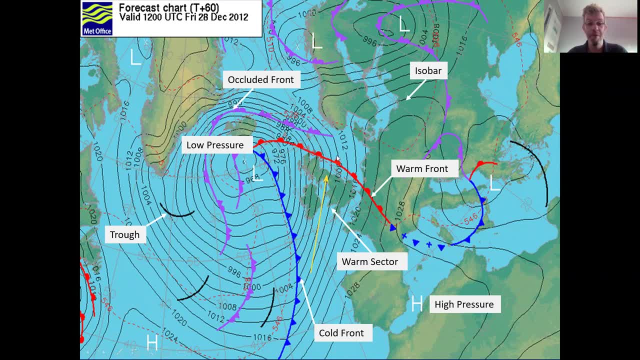 this cold front pointing that way, We've got this warm front pointing north. At the same time as these kind of fronts are moving, the whole low pressure system is moving anti-clockwise And a little bit of kind of background information here. All the low pressure systems can. 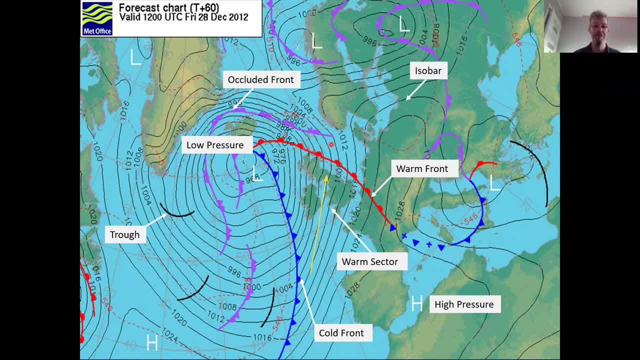 kind of form in the southern part of the Atlantic and track across the UK towards us. So they move from the southwest to the northeast while they're rotating. We can tell a number of things from this, And I'm just going to come back with my little 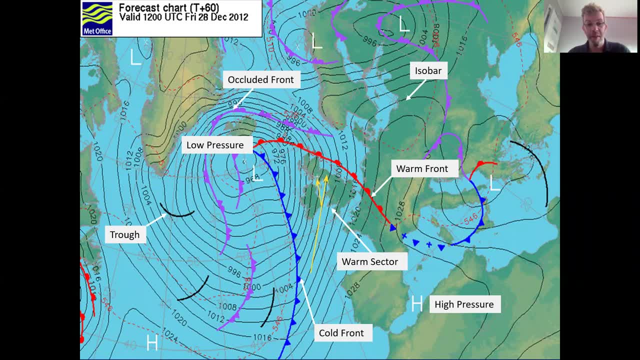 yellow pointer And you can see if I draw a couple of lines on these synopses. it's about lines, the isobar lines. we can start to get an idea of what the weather's being in the wind, And the wind's the crucial bit. 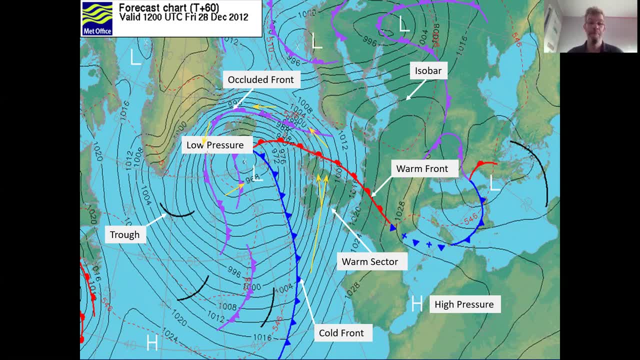 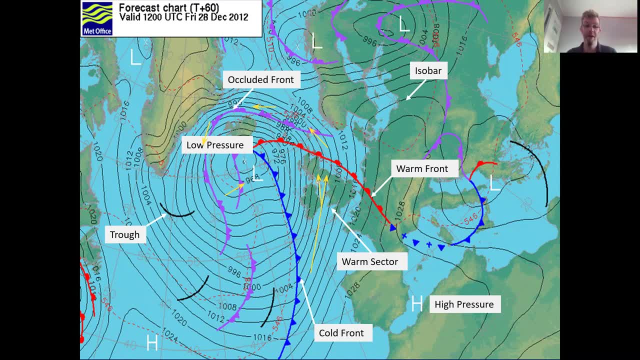 So that's why we've got a line here. So that's why we've got a line here, And then we've got the second arrow coming off. The reason for this is the low pressure creates a vortex that pulls everything into the middle. 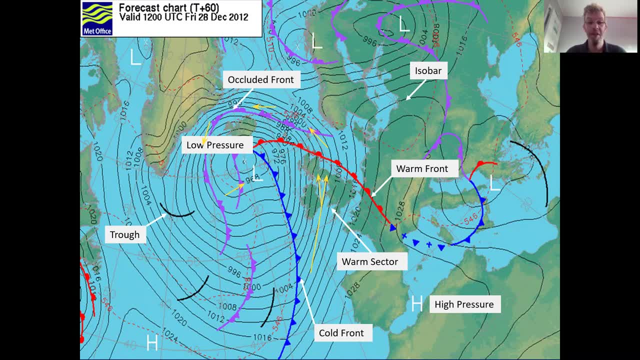 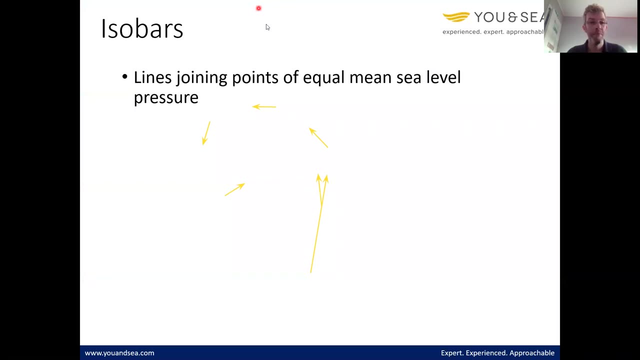 So that will give you more of an accurate wind direction at the location in which you're on the water, And we'll come back onto this in a little bit more detail. Okay, a little bit about a recap of what we've got. So: isobars: joining points of sea level pressure. 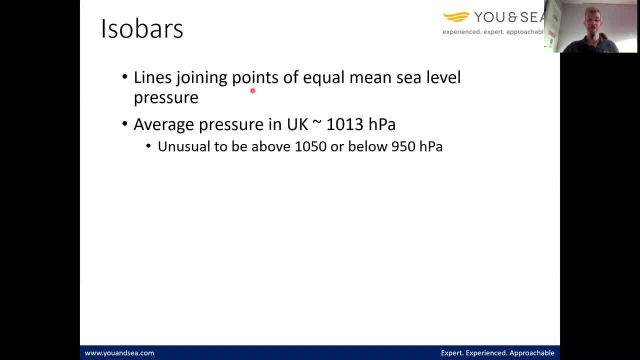 about 1,013 is the UK average pressure. Anything below that and we're generally going to be looking at low pressure territory. and anything above that we're going to be looking at high pressure territory As a side note and we're going to listen in a bit more detail. 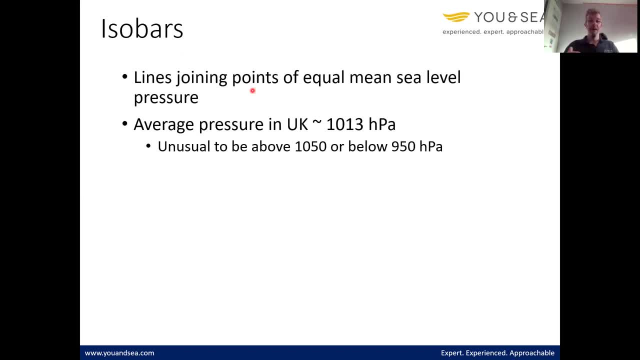 when we start talking about tides on a different video. as the pressure drops, so a low pressure gets moved into the UK that pulls the water level up As a high pressure moves in that pulls the water level lower And that in some cases significantly affects flood defences. 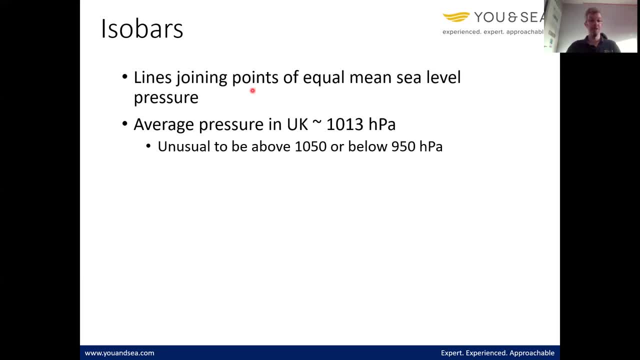 going under bridges. It can also affect tidal water if you are operating in an area where there's lots of fresh water in addition to tides. And the best example is two examples close to where we're based in the Clyde. One is the top of the Clyde at Glasgow. 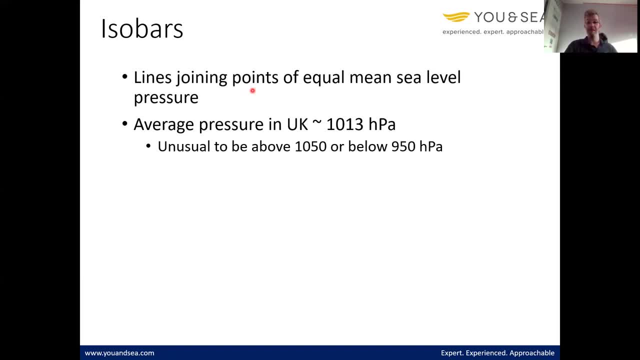 We were recently up there doing some filming and for the first seven hours we were filming we'd just started at the turn of low water. so we're at about six, six and a half hours up to high water And the water level was rising. 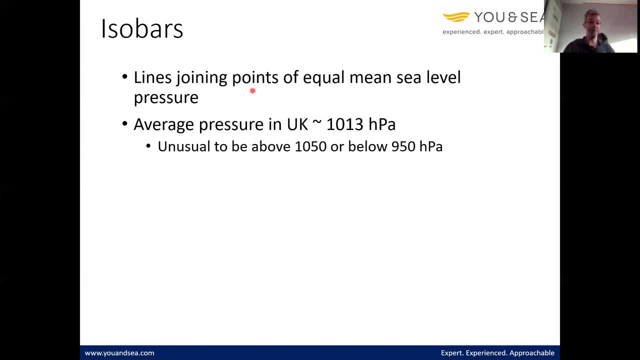 but the very surface current was going back downriver as if it was simulating an outgoing tide, And this was because there was so much fresh water further up river from all the rainwater we had. The other location is Loch Lomond. 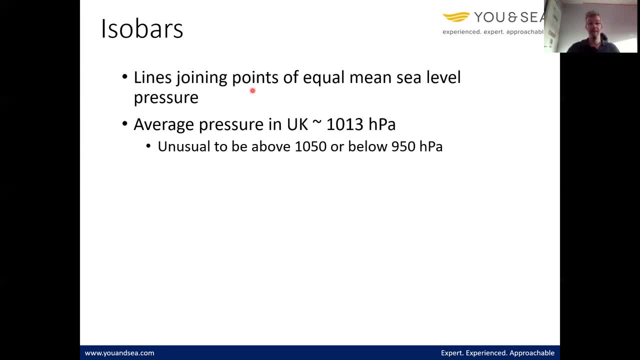 which, in the very bottom section of it, is a tidal location. It does go up and down quite dramatically. It's affected much more, though, by rainwater and low pressures and high pressures, And the further you go up to the north of Loch Lomond. 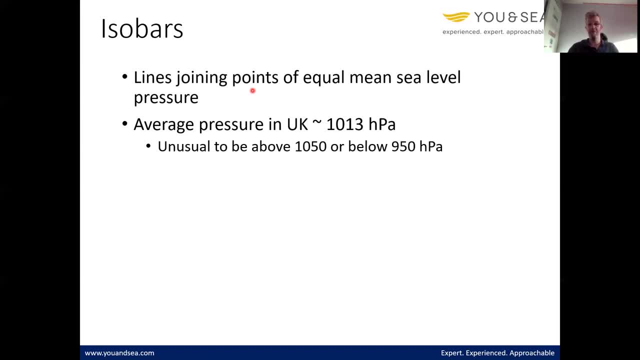 the more. that is very evident And the water can move by about two or three metres depending on how much rain has happened or is happening. So we can use an isobar to identify wind speeds and wind direction. We can see instantly where the high pressures are. 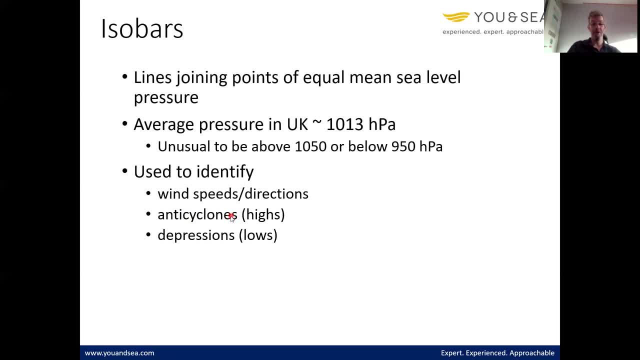 and that's what we call anti-cyclones, And we've got low pressures and what we call depressions, And we can also pick out troughs as well in black lines, Ridges, kind of a ridge of high pressure moving in. 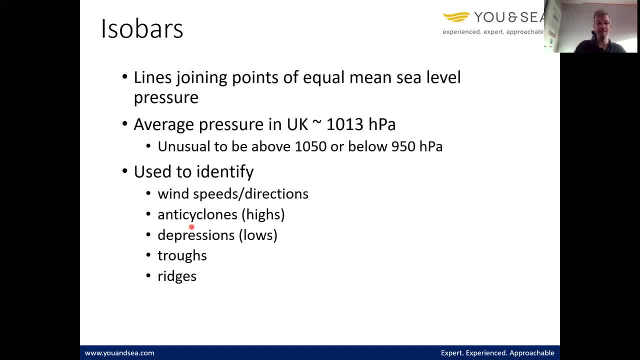 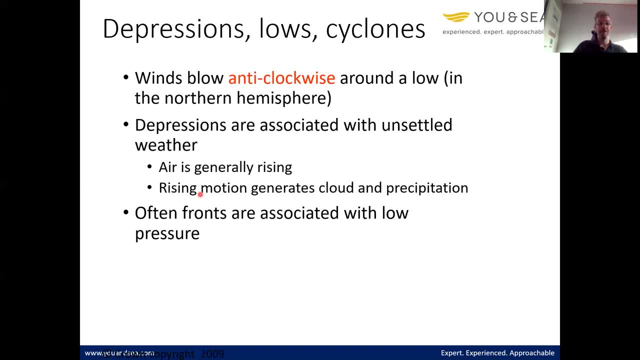 that's what we call that. But keeping it simple for now, we've got anti-cyclones, high pressures and depressions, low pressures. So instantly let's start talking about a depression- aptly named- Depressions and low pressures. 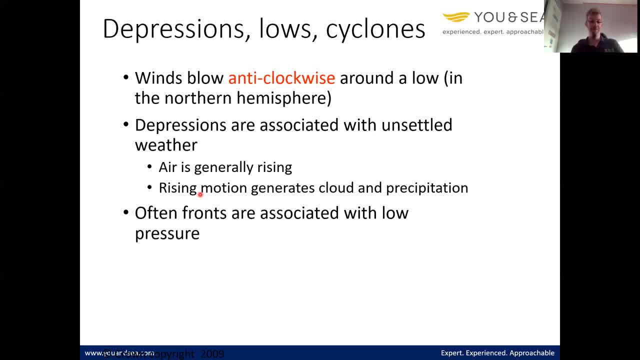 It's windy, it's wet, it's changeable- Three words to describe a low pressure. Anti-clockwise around the low pressure in the northern hemisphere. Round about the low pressure, the clouds are going to start to play a factor And it's really quite easy to see a depression coming in. 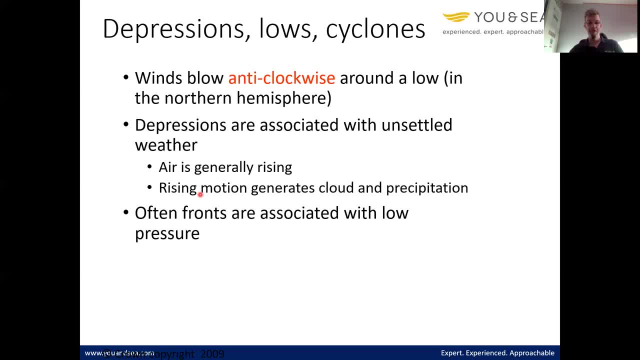 because the clouds will change And I'm going to record a video on clouds and upload it as well to our YouTube channel so we can chat in a bit more detail about what clouds do. But the reason we pay quite a lot of attention to what depressions do. 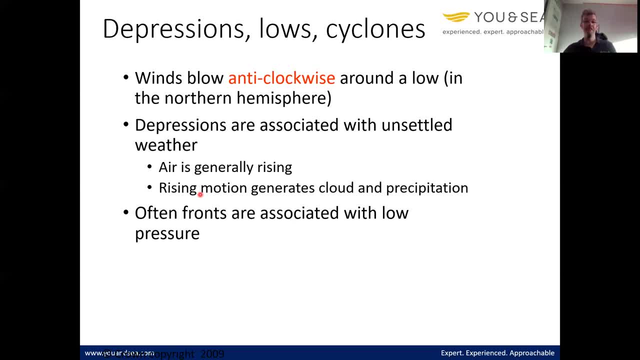 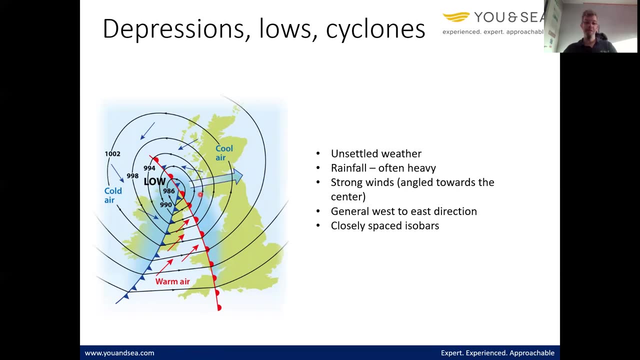 is because they bring wet and windy weather and an increase in sea state and an increase in humidity, And they also increase in water level as well. So, as a recap on depressions, we've got unsettled weather. It's very changeable. 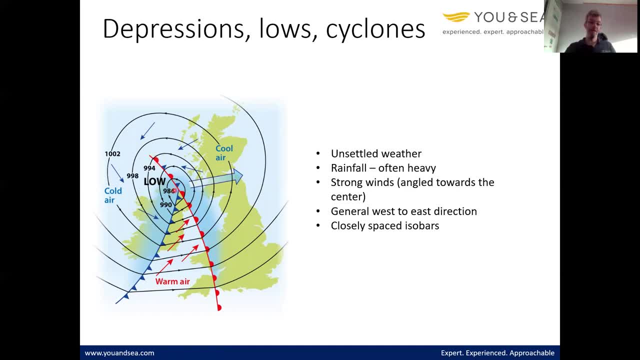 This is a picture one, but it kind of depicts very nicely what happens on our occluded front here, where the two have started to sit together Anti-clockwise rotation. We've got a warm front, kind of leading down the middle of the Irish Sea. 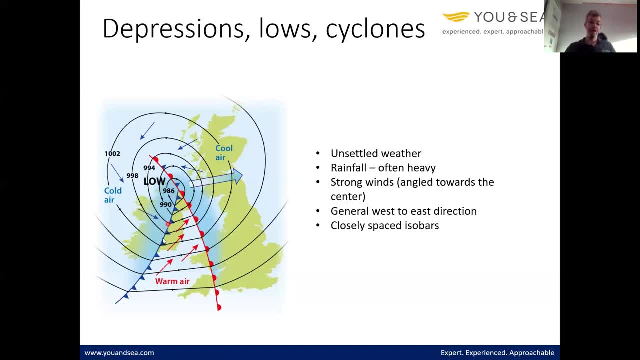 Warm section in the middle, And then we've got our cold front, which is sat across Ireland at the moment. As always, a west of east direction, Tightly packed isobars, Strong wind, Kind of vortex into the centre of the low pressure. 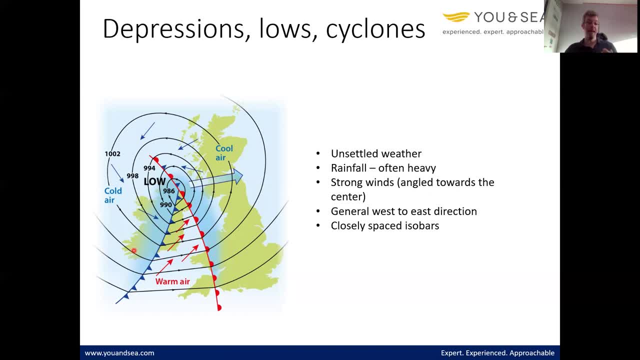 And as it says in the second bullet point, there it does bring a vast amount of rain And that rain, across the passage of a low pressure, changes from very light drizzle to gradually kind of heavier, more persistent rain. The middle section here. 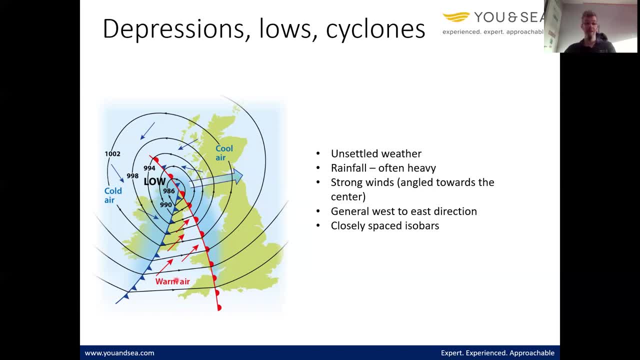 the majority of the rain is passed under the warm front, So in the warm sector we tend to get drizzle. And then, as the cold front approaches, the drizzle tends to become more kind of squally isolated showers. And then the squally isolated showers. 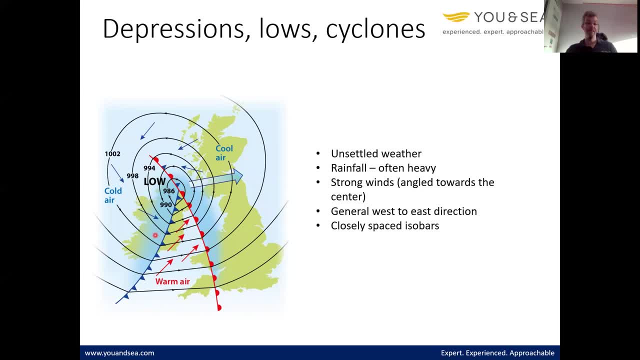 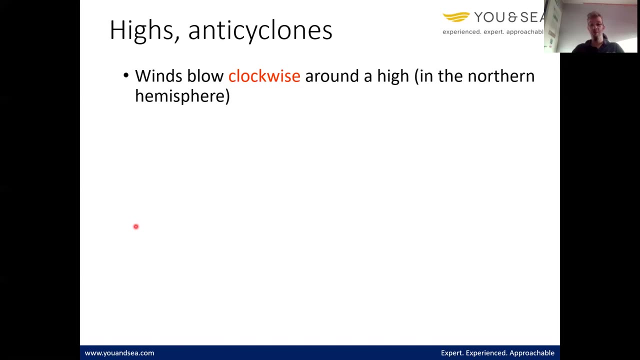 will get less frequent, less heavy, as their system passes away. And we end up over here in relation to the low pressure. So high pressure, We're getting some nice weather, So it's clockwise. Northern hemisphere again. remember Anti-cyclones, even though they spin clockwise. 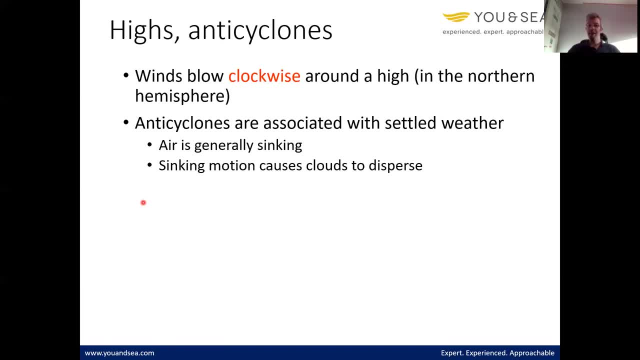 generally get more settled weather And even in the middle of winter a nice big high pressure. although it will be reasonably cold, it will be sunny, And you tend to get that weather for about a week or so until that high pressure kind of fizzles out. 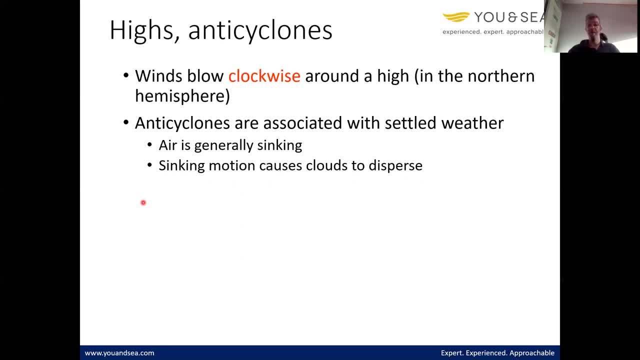 and the next low pressure moves its way in And we're never too far from a low pressure in the UK. Nice and sunny, warm weather in the UK In the middle of summer. frost, fog, cold, dry icy in the middle of winter. 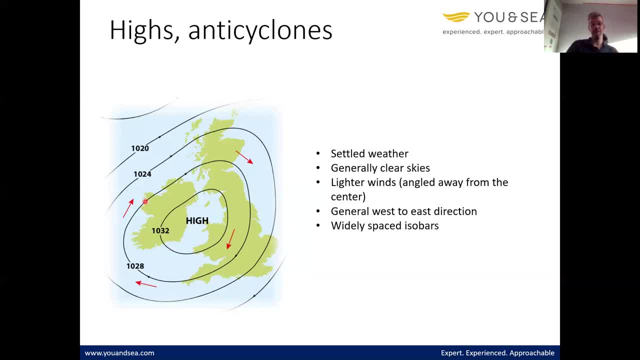 You can see from this photo that high pressure looks very different. There's a lot less stuff moving on here. We've got isobars that are relatively spaced. It's not very windy. There's no fronts hanging all the way down through the UK. 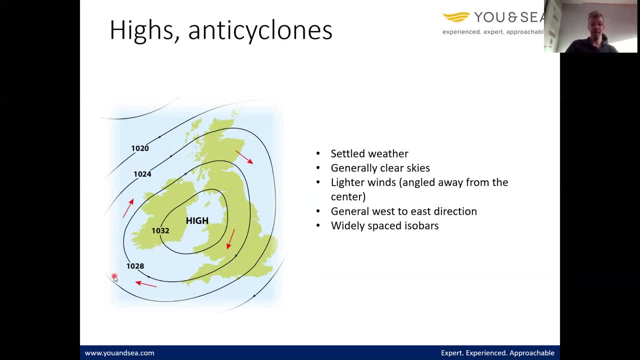 There's no cold front over here, So there's generally a lot less happening. So we can summarise at least points there very nicely Settled and it probably will be for about a week On the whole reasonably clear skies. 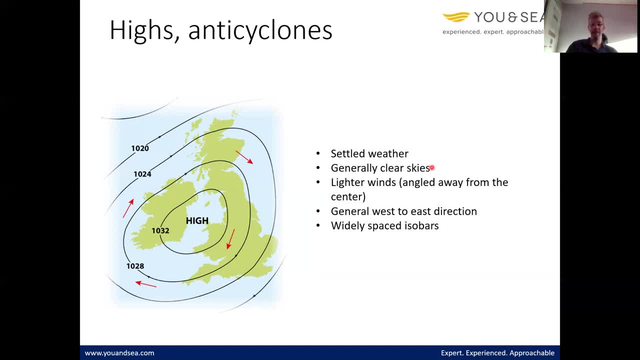 But let's not rule out fog and everything that occurs with fog- And I'll talk about that in a later video. It's a wind angled away from the centre, So it's trying to disperse the wind, which is why we get lighter winds. 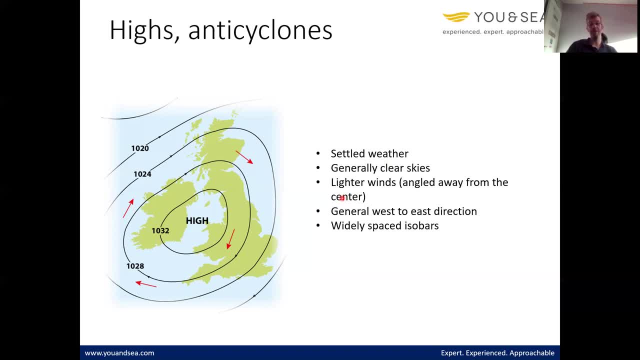 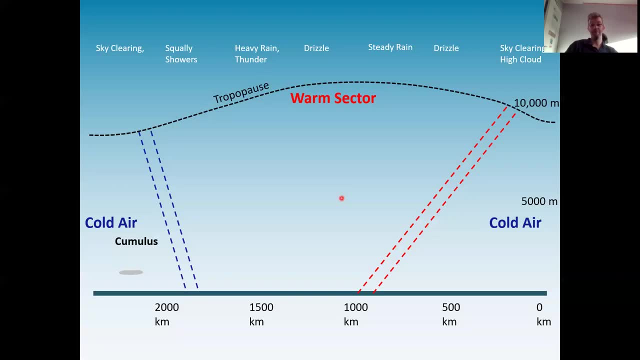 Again kind of generally a westerly, generally a west to east- And I'll move in from the Atlantic and sit in the UK for a while- And widely spaced isobars. So this is one little kind of cut through of a snoptic chart that I come back to. 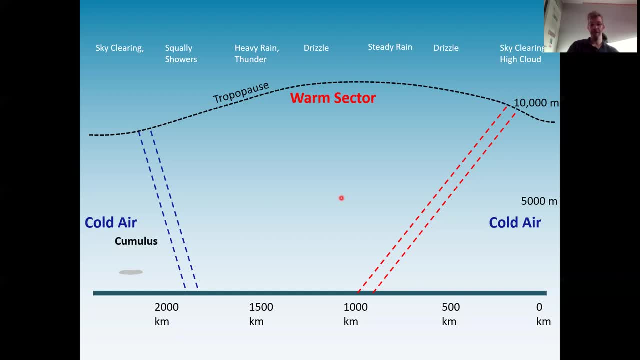 time and time again on shore-based courses, And it's really quite good because it lets us see what is happening and try to kind of imagine it. So right up here, take a nice summer's day, blue sky, and we'll get some kind of indication. 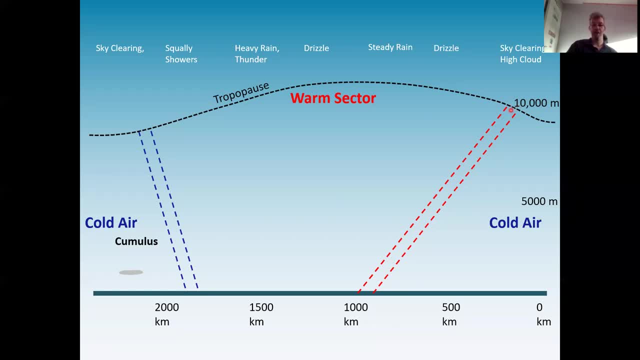 that the weather's going to change, Whether that be a forecast or simply looking up at the sky and going: hang on, there's a few clouds up here. Let me have a look at my app on my phone and see what's happening. 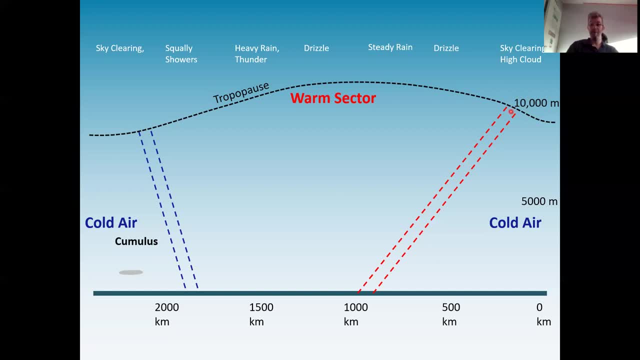 And it could be the next day that the forecast is going to be pretty wet and pretty windy And it's going to take the rest of that day and night for that low pressure to move in. So what we can see from starters is the warm air is rising. 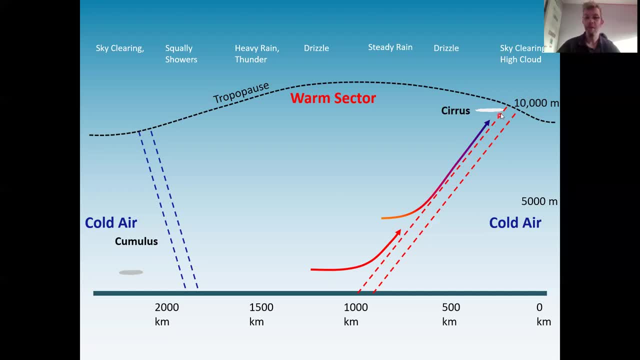 That's what these two lines are indicating. here We've got cirrus clouds. high, thin kind of crispy strands Start to move to kind of more layered clouds. Anything that's got a stratus in the name is a layout, So a cirrus kind of high frozen layer of cloud. 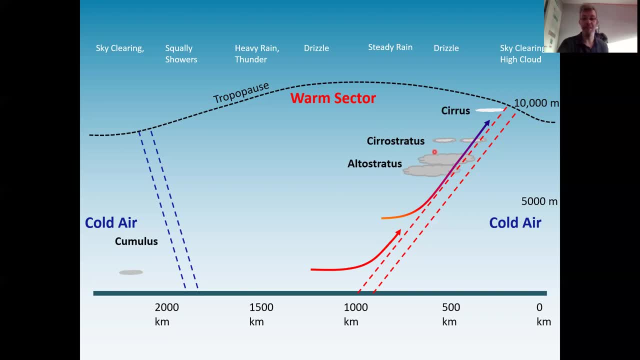 Alto stratus just starting to lose the frozenness of the cloud, but still starting to layer, And at this particular point we start to lose the sun. We throw in a couple of alto cumulus clouds, So they're starting to kind of heat a little bit. 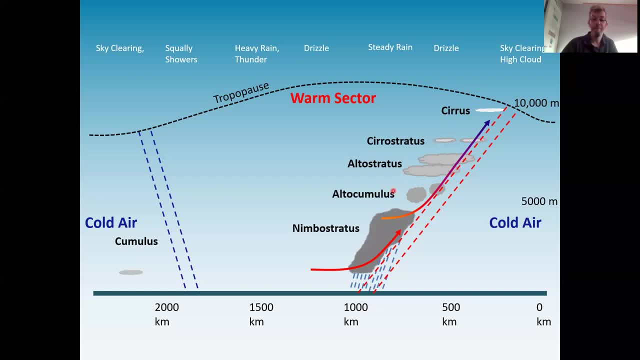 Thing to do with heat. clouds is going to mean rain. Nimbus stratus follows- And this is the crucial bit, because this is just after the warm front hits, which is on the warm front, And nimbus stratus clouds are really heavy, persistent rain. 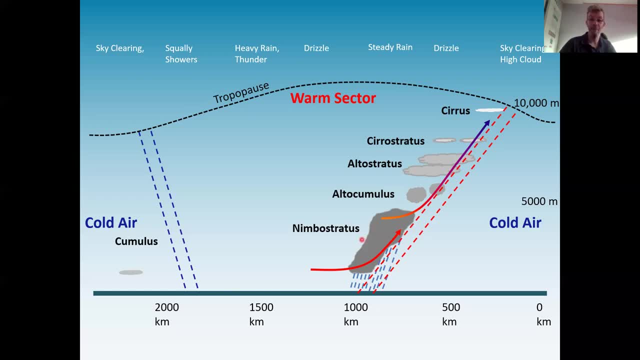 It's a wall of rain going to move across as that front passes overhead. The good news is the rain is not going to last forever. Still here, this is what we call our warm sector. We've got a stratus and we've got stratusy clouds. 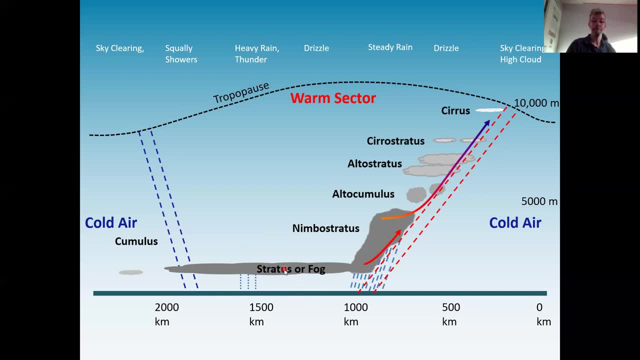 And that could turn into fog depending on the visibility. The crucial bit is we've lost the nimbo from the name, So we've lost the rain element of it And they're literally just low lying clouds. It's a bit of drizzle, bit of mist. 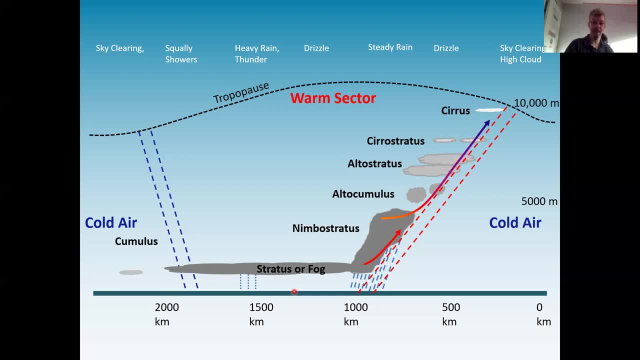 not a great deal else happening in terms of cloud and rain anyway, And then it all changes. So then we get the cumulonimbus cloud And this is the towering thunder cloud that brings all kinds of funky weather Cloud. you're most likely to get squally showers. 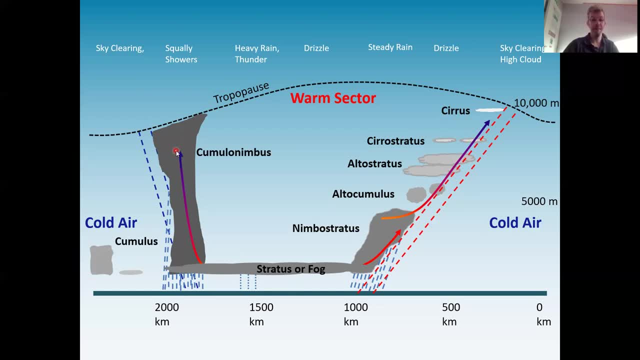 Possibly thunder and lightning, depending on the time of the year. We could get thundersnake, depending on the time of the year as well, And also hail or any one of the above together. Why do we get this? Because we've got warm air over here. 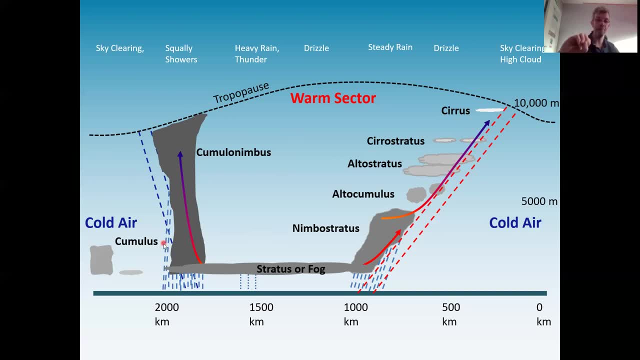 and cold air suddenly moving in behind it and forcing it up quite rapidly, And that forces it into kind of a tumble dryer effect. It's rising, cooling, dropping, and then meeting the next kind of influx of warm air And it turns into reasonably violent battleground. 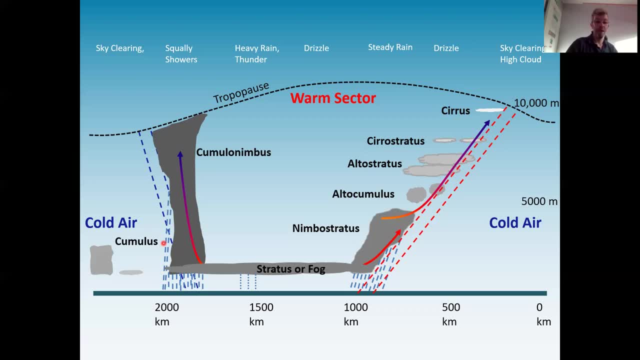 which is why we get the thundersnow and the thunderstorm In addition to those clouds and everything else that goes on within the cloud. what we see under here, under the cloud, is generally heavy, squally showers. It's not heavy persistent rain. 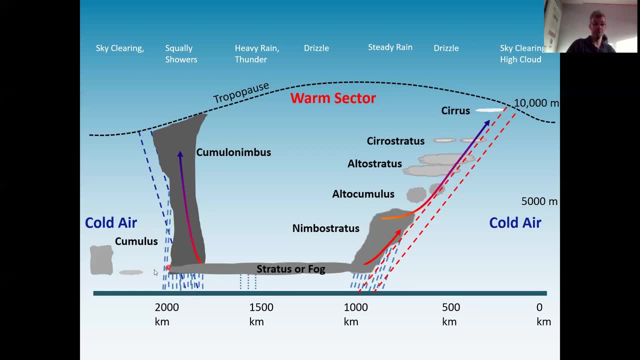 like we get over on the warm front: Squally showers that will stop, but it will build up again and the next squall will come through. And then the good news is that's the two fronts past, And then we are going to start to look at cumulus clouds. kind of the white fluffy clouds. On one hand that's good because it shuts the door to one light pressure system. On the other hand, it's bad because the pressure's risen again, which opens the door to the next pressure system to work its way in. 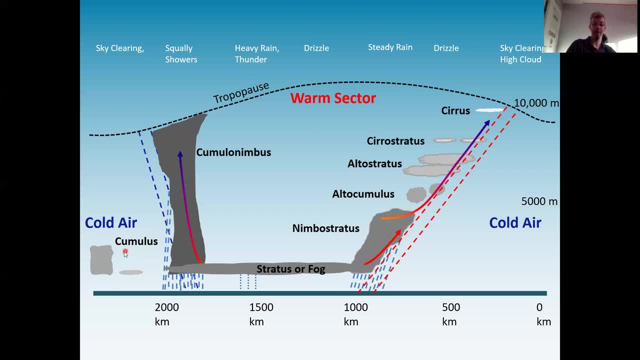 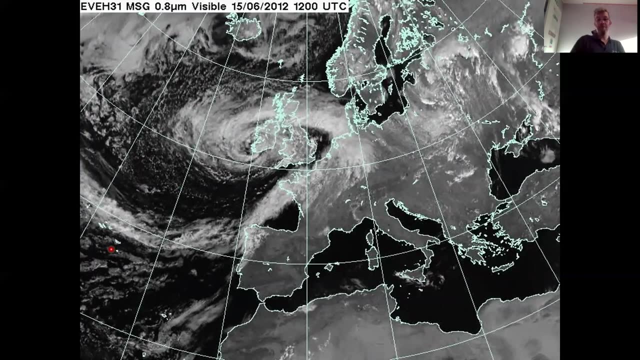 But there is a period here where the weather is generally quite nice. Last slide for this particular PowerPoint. This is an overview of a low pressure system showing the clouds, And we can quite quickly, if I've got a tool in yellow, just bring it out. 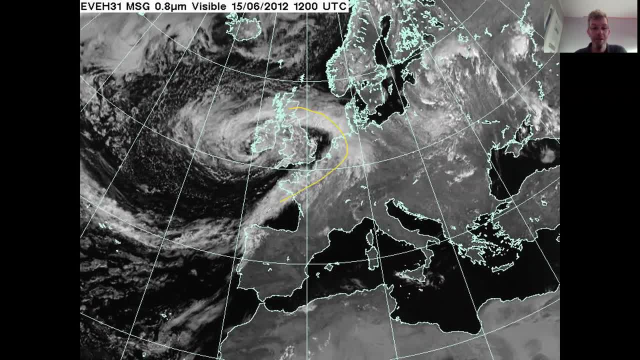 What we've got here is one system going down there and it probably extends all the way around here, But it's this little bit that we are interested in, True synoptic chart styling. Let's redo that And I'm going to colour it red.